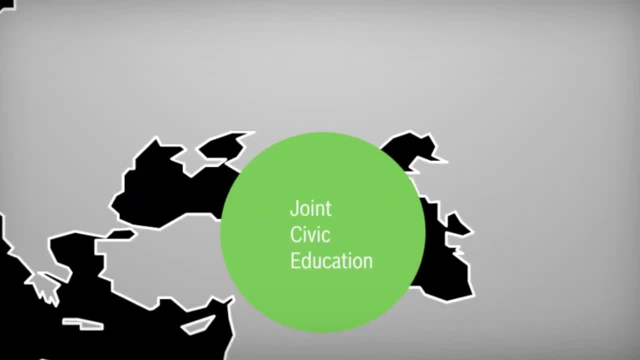 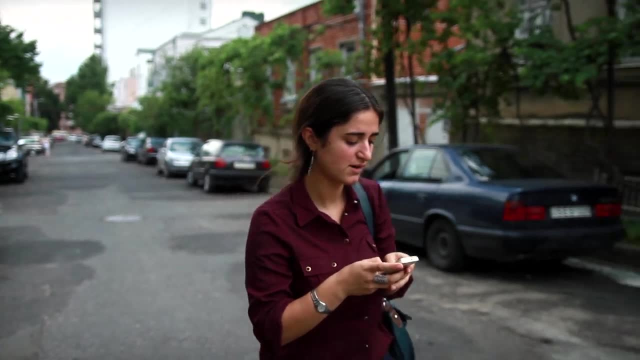 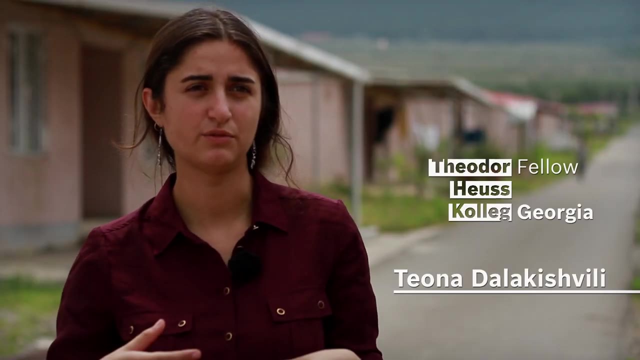 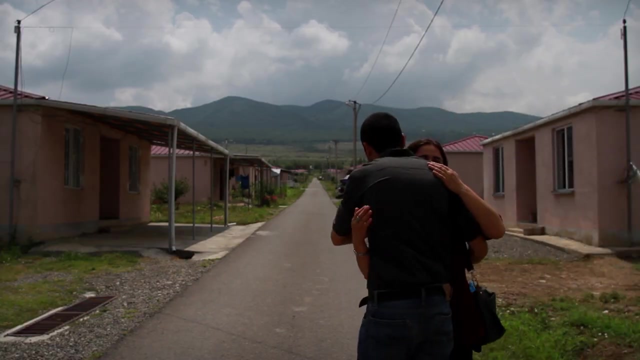 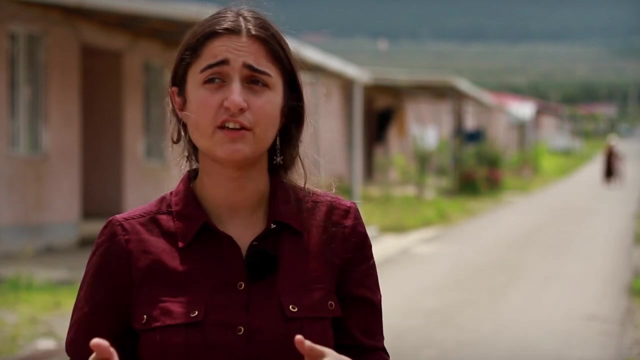 After the war happened in Georgia, all people get somehow active and we're helping these internally displaced persons, But after like one month everybody forgot that these people still existed. They had still problems. And after one year these problems were even bigger for these who live here, because they are separated from all other settlements and they are somehow 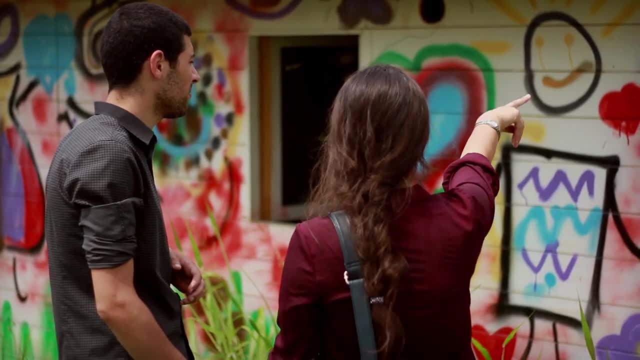 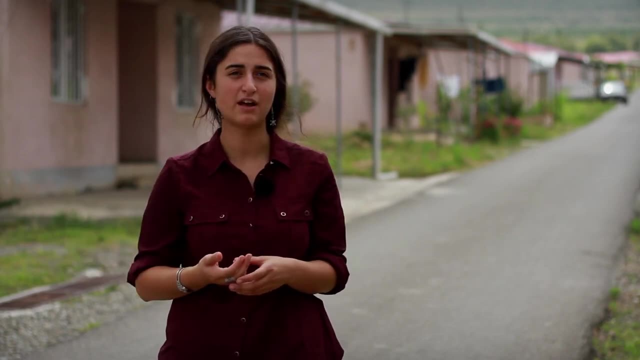 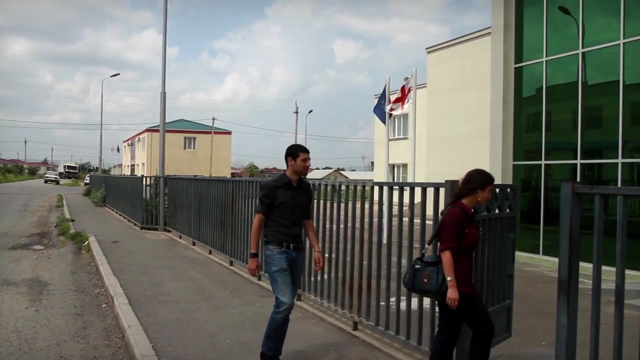 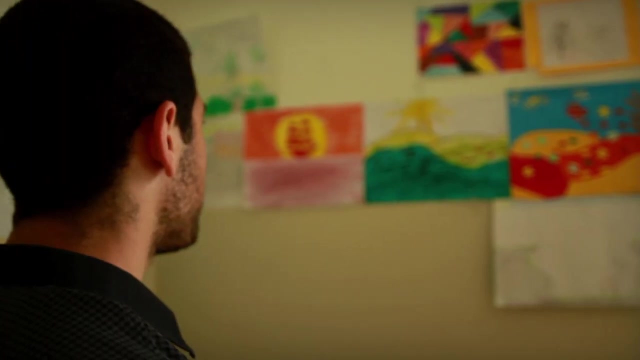 becoming a closed society. The children: they have this lack of having a playground. They did not have some art classes at school, Or if they had, this problem was that the price was very high. We wanted to do some art classes for these children and we have. 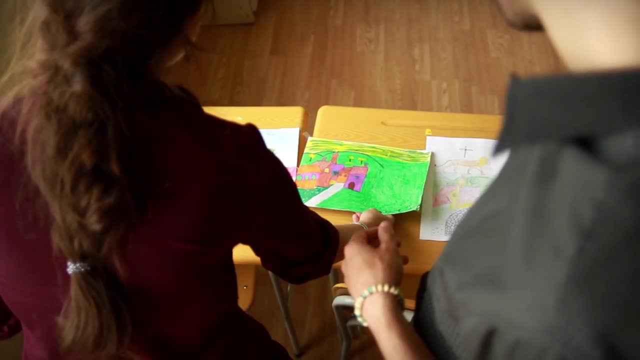 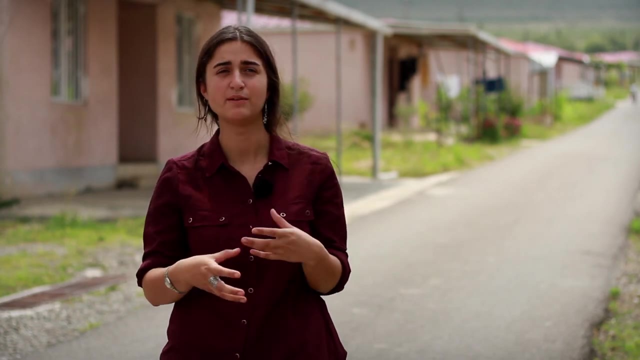 done this project: the art days. We were coming here for approximately 2 months every Sunday at the school. then we collected the paintings There. we were making also the handmade jewelry and we had a quite nice big exhibition in Tbilisi. And with this money, which was children's- money, because it was those people who had the money. they were constantly singing and Mai Ho lev it like an afternoon song in Tbilisi And we were able to gather a lot of money. Thank you, Moise, for taking this show and position as Roza cue to tell us why it is así, for that. 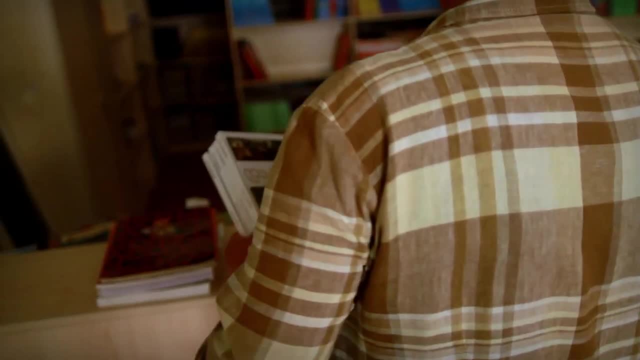 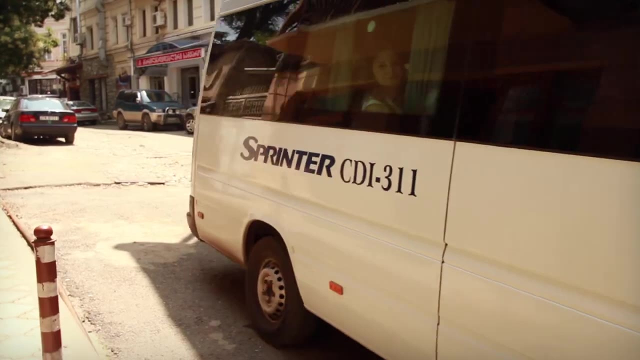 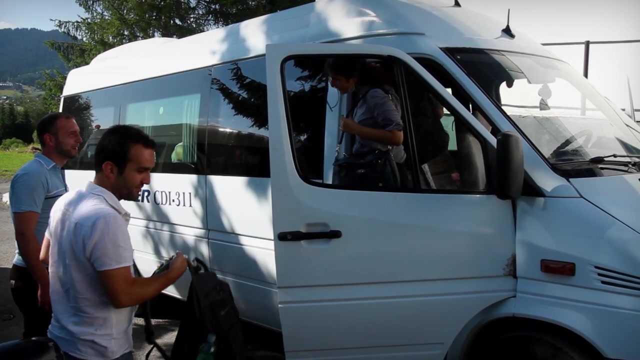 It was their work. we bought these books and we made this art corner at this library. The idea itself existed in my mind, but the Darhuis Collect helped me to realize I should not wait, I should start moving and I should start making something, some action. 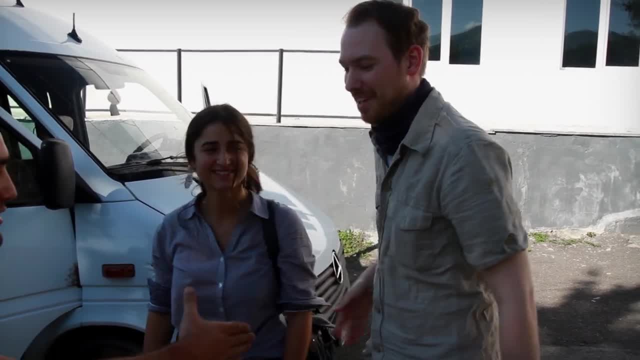 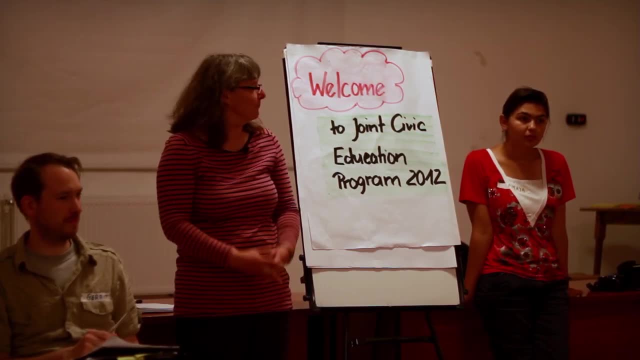 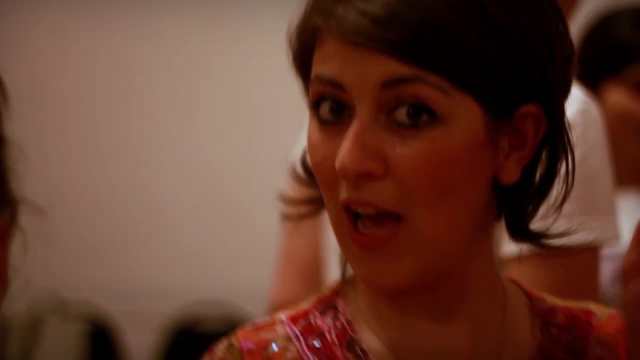 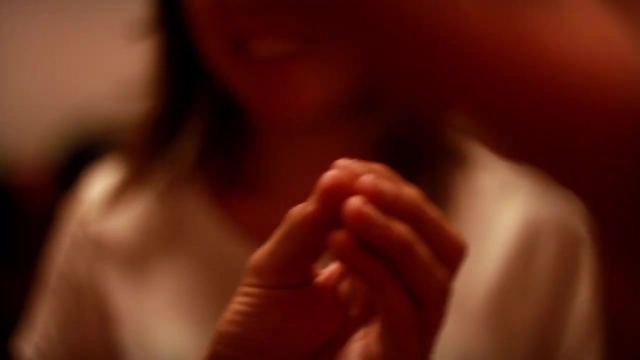 So it was always with the countries of Armenia, Azerbaijan and Georgia, and the new ones are from Turkey and from Russia. So welcome very much here in Bakuriani. My name is Ahmed. I'm from Turkey. in Istanbul, My name is Anna. I come from Armenia. I live in Venezuela. 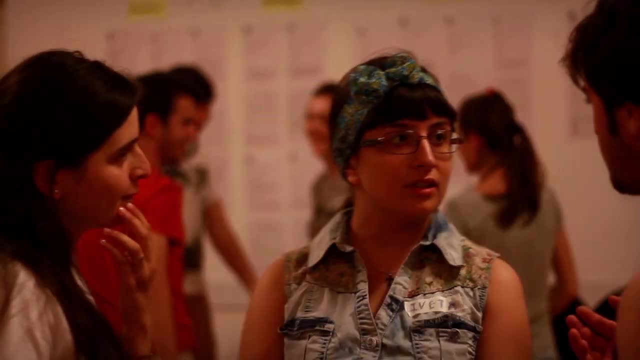 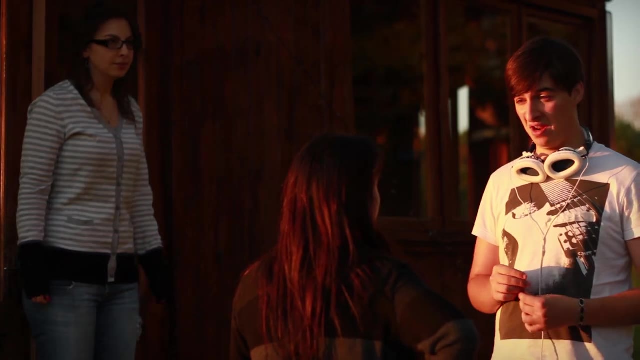 My name is Belashah Mirza. I came from Karachay, Circassia, it's the northern Caucasus of Russia. I'm Jehun and I come from Azerbaijan, from the Ganja, second largest city. Capacity building in our project means that.